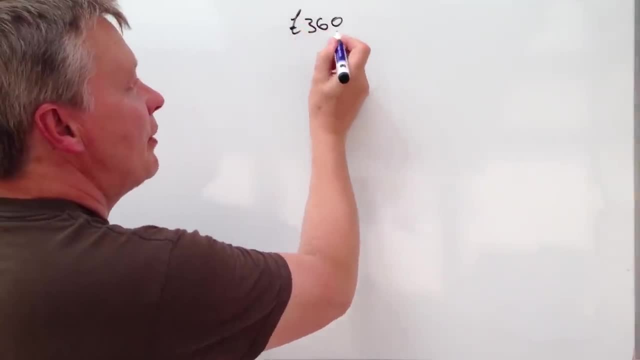 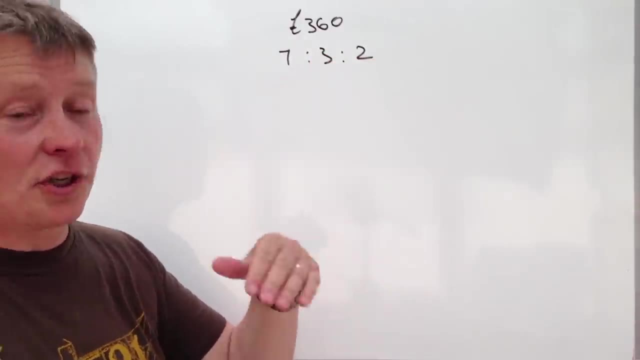 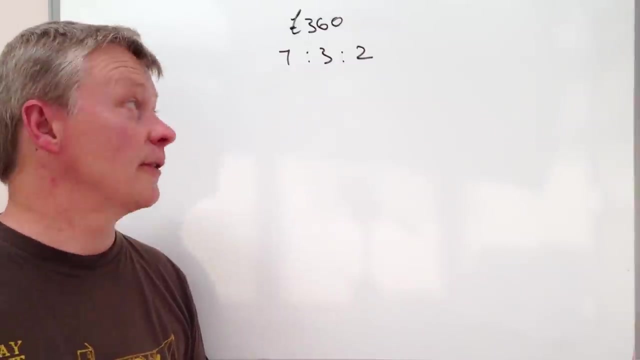 looks at sharing £360 and it's in the ratio 7 to 3 to 2.. I will put the question just below in the description box, or you can visit mathsrapcouk and that will give you quite a lot more information. So somebody's won an amount of money on the lottery they've 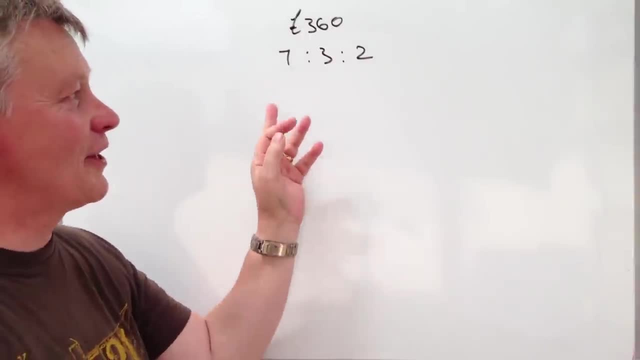 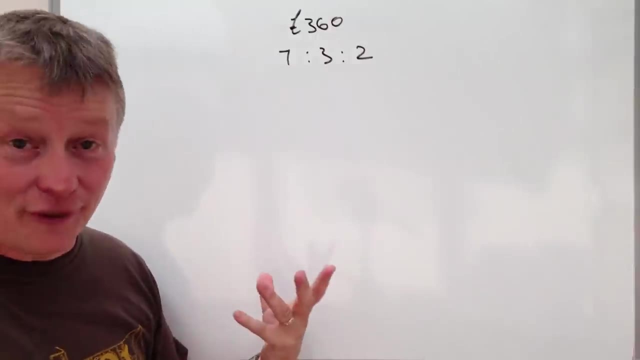 won £360 and they're going to share it in the ratio 7 to 3 to 2.. Okay, and the question wants us to calculate how much the person who gets seven shares how much of the pot of £360 they actually get. Okay, so if you're sharing things in ratio, the main issue with 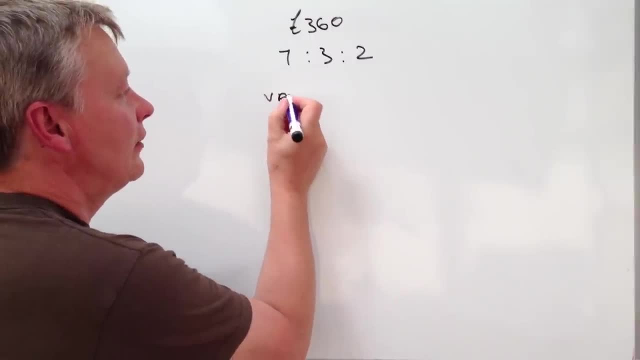 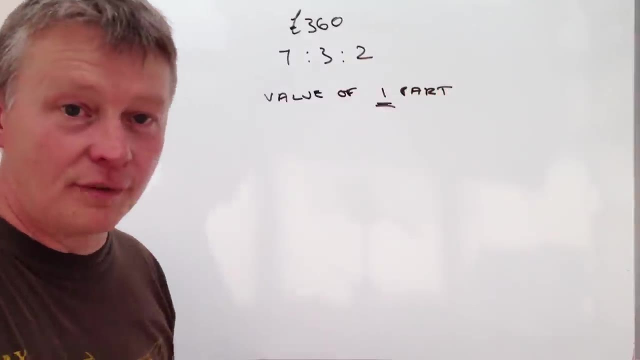 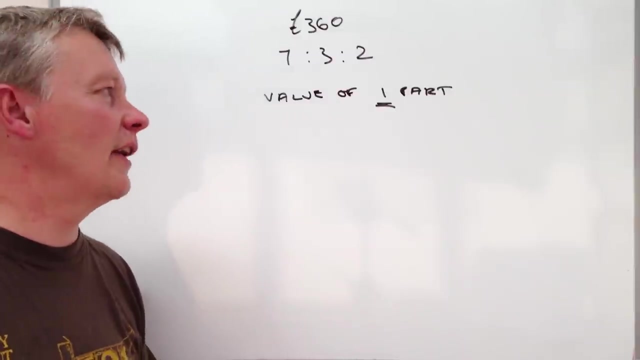 it is, you need to find out the value of one part. Okay, that's the most important thing with ratio questions And really most of the ratio questions, as I mentioned, fall into largely the same sort of area. So, provided you find the value of one part, then it should. 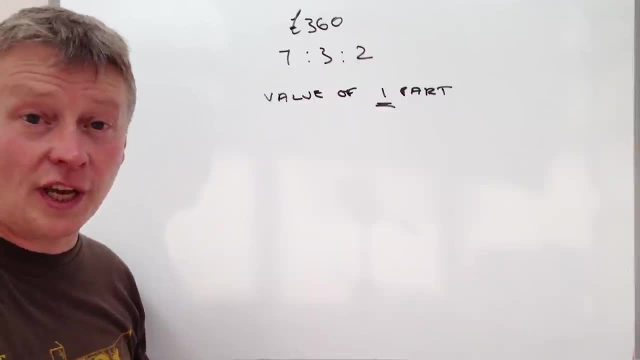 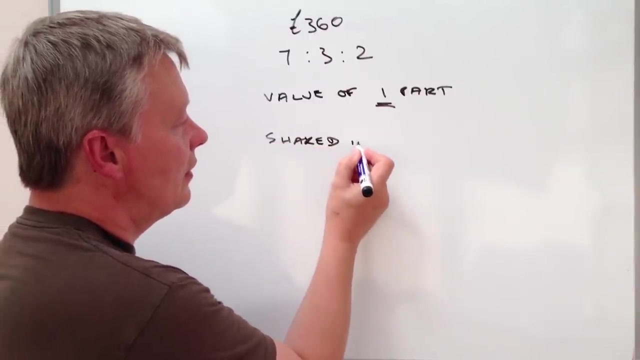 be relatively straightforward to work out the value of each of the share values. Okay, so in this particular case, what we've done is we've got £360 and it's actually been shared into. so it's been shared into 12 parts. Okay, because we've got £360 and we've got 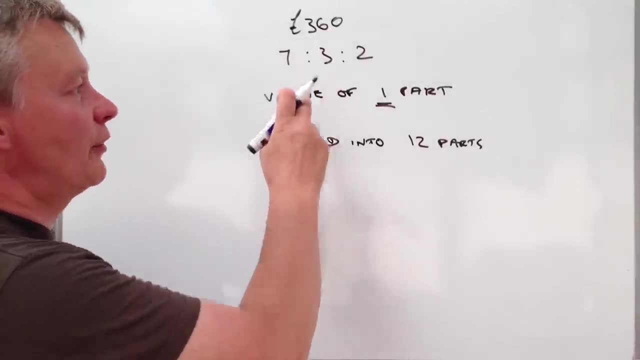 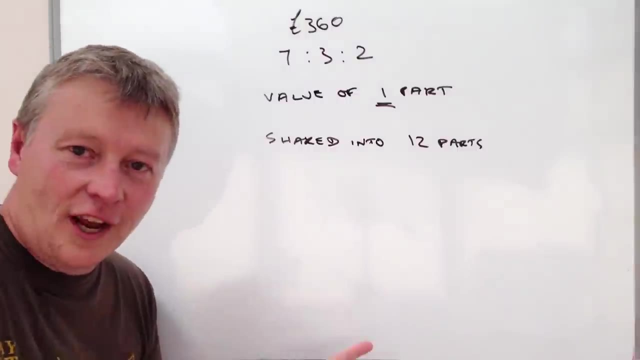 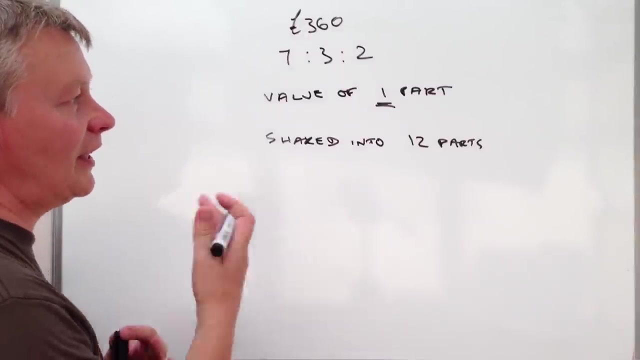 £360, somebody's got seven parts, somebody else has got three parts and somebody else has got two parts. If you add that little lot together, then in order to share out the whole £360, then 12 parts have been given away. Okay, so, in order to find the value, 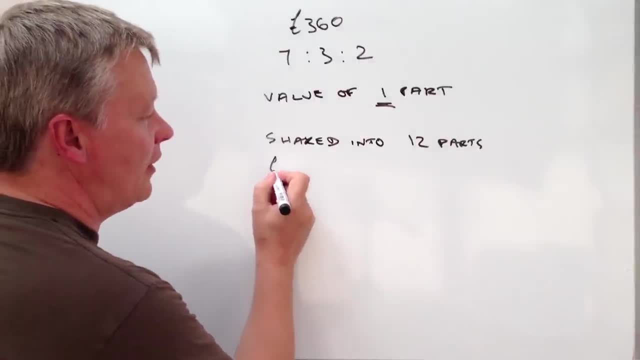 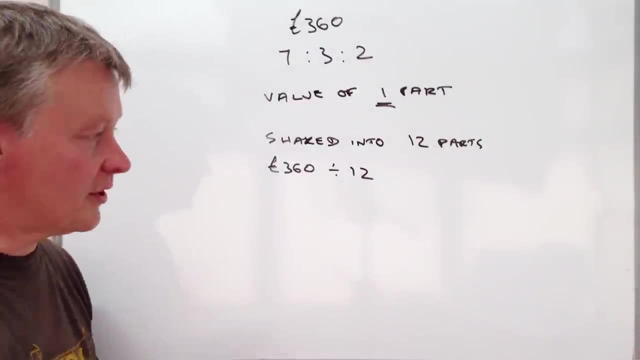 of one part. what I'm going to do is I'm going to divide £360 divided by 12, and that will give me the value of one part. So in other words, if I've got £360 and I've got £360, then I'm going to divide £360. divided by 12, and that will give me the value of one part. So in other words, if I've got £360 and I've got £360, then that value of one part should be over £250 and that leaders확eree gets the TP value. Okay, Now, in order to test whether that's true or not,